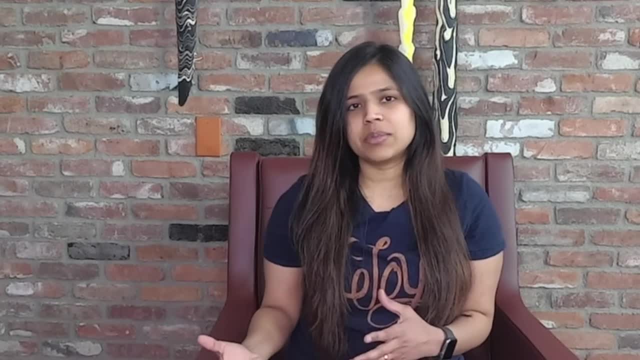 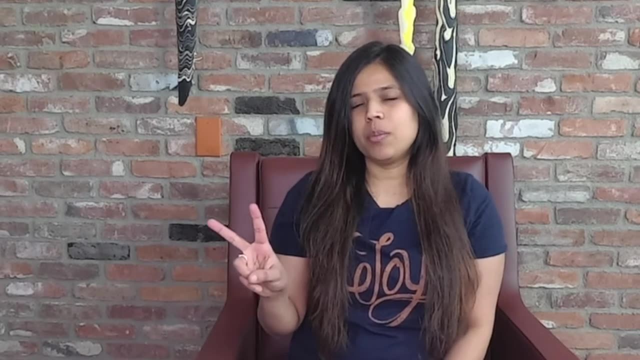 the field of robotics. Based on all of my experiences, I'm answering the question: what are the skills required for robotics? I'm going to answer this question in two parts. The first one is about the skills required for robotics and the second one is about the tools. 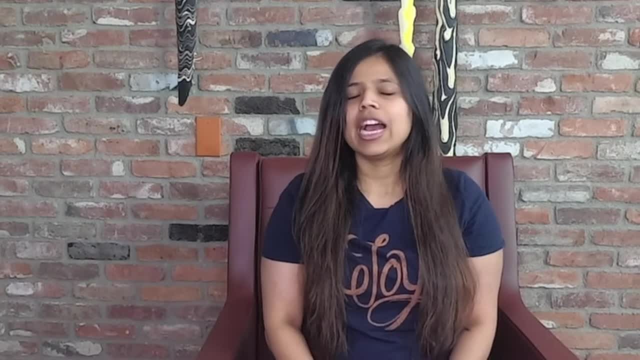 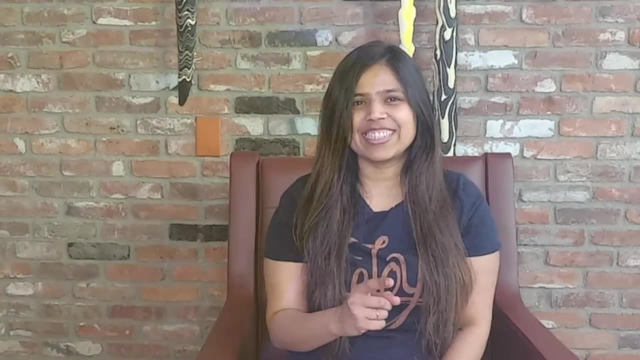 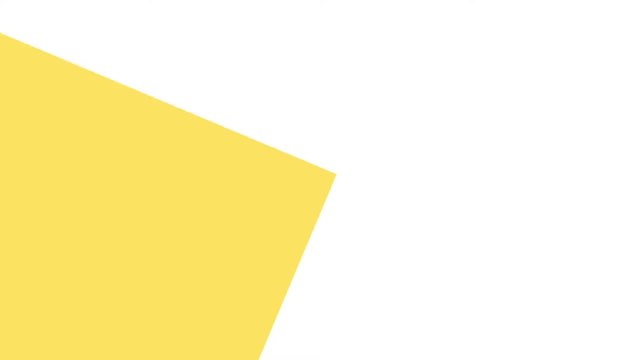 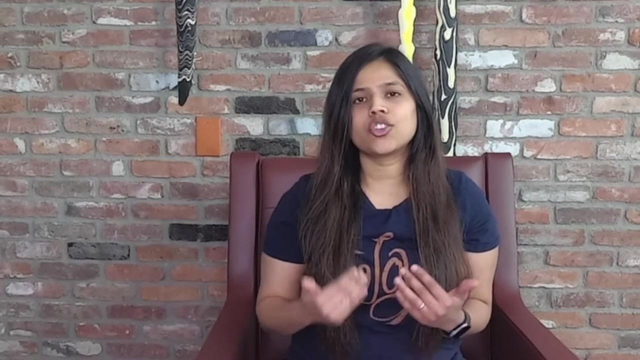 and technologies that are helpful in the field of robotics. I'll include all of the timings and useful resources in the description below, So without further ado, let's get into it. I'm a robotics software engineer, so I'll be answering based on the software perspective. 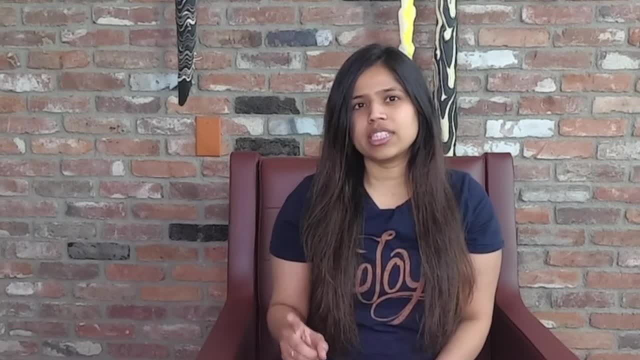 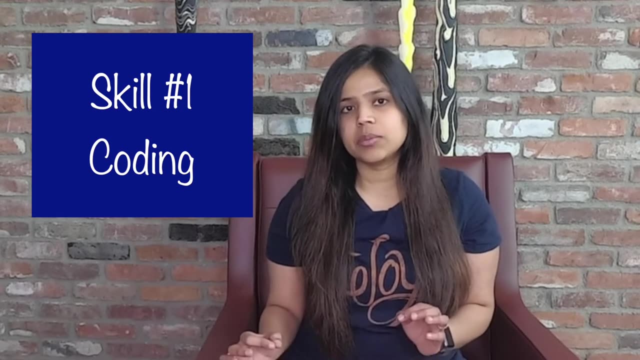 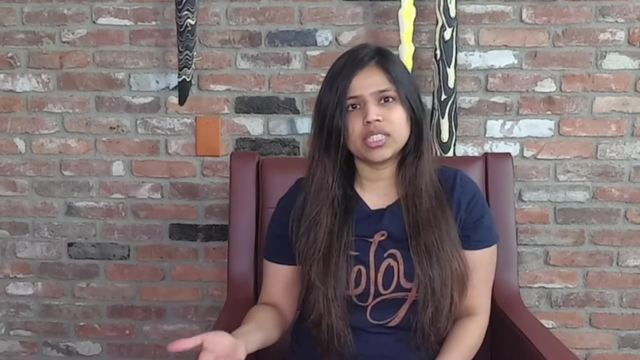 Having said that, the number one skill you need for robotics is coding skills. When I say coding skills, you don't need to learn just print an if else statement. You really need to learn how to code. This includes writing functions, classes or other object-oriented principles. Now basic. 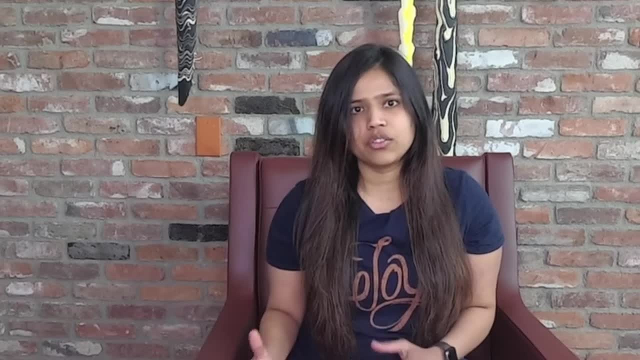 robotics can be done with just if else, statements, But if you want to learn how to code, you need to, such as a line follower. However, if you want to advance in the field of robotics, you really need to learn how to code. 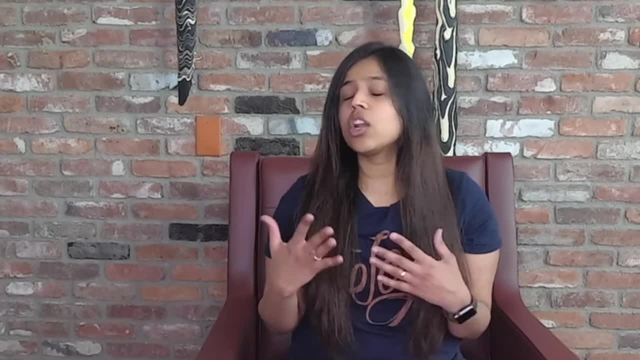 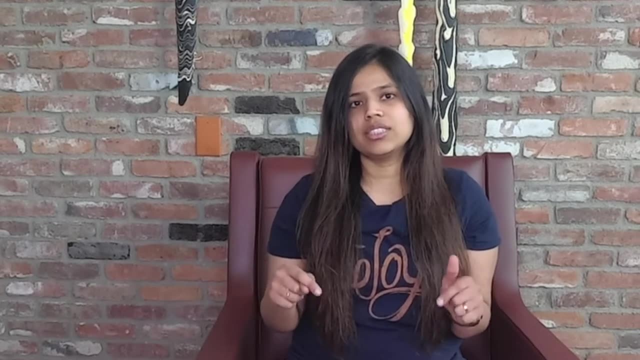 I would recommend take a little bit of time and learn how to code. There are lots of useful resources. I personally use the New Boston YouTube channel to learn how to code. I'll include it in the description below. The second skill you need to learn for robotics: 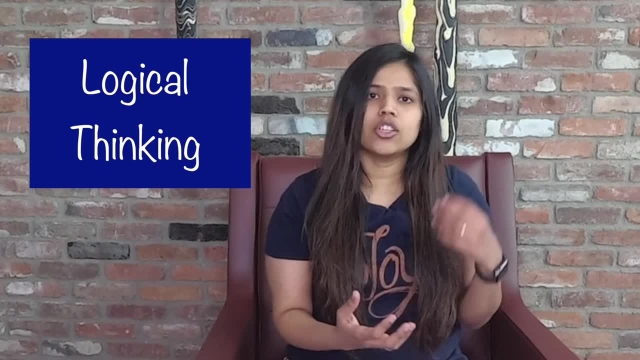 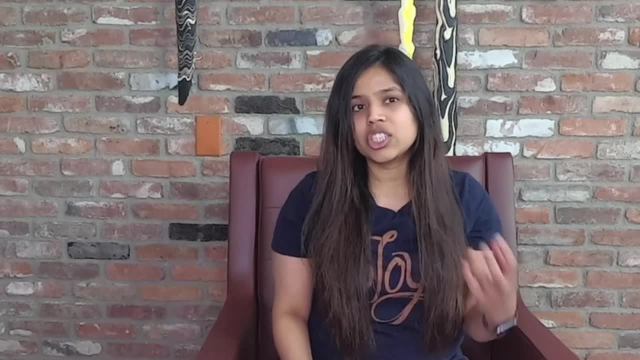 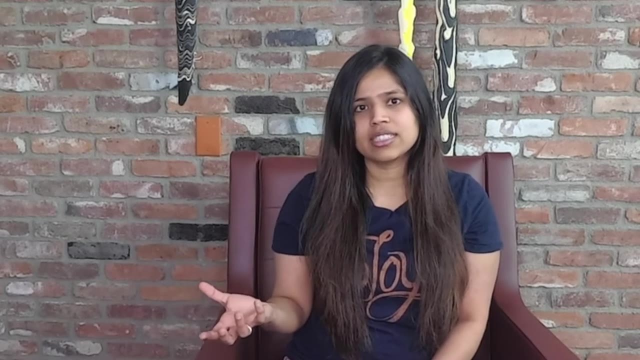 is logical thinking. Just like with speaking, you have grammar and words. that is syntax in programming language. But to formulate your thoughts and articulate you really need to be thinking. That is what logical thinking is for programming and robotics. In other words, you need to know how to solve a problem. 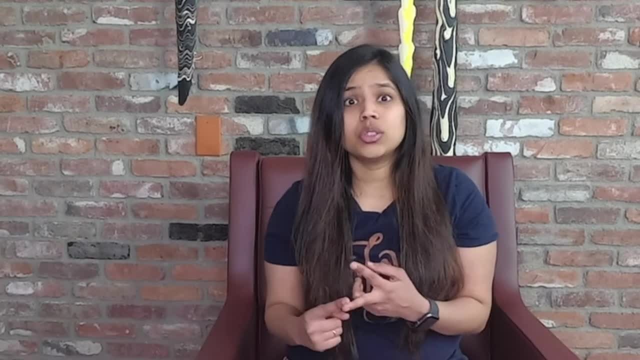 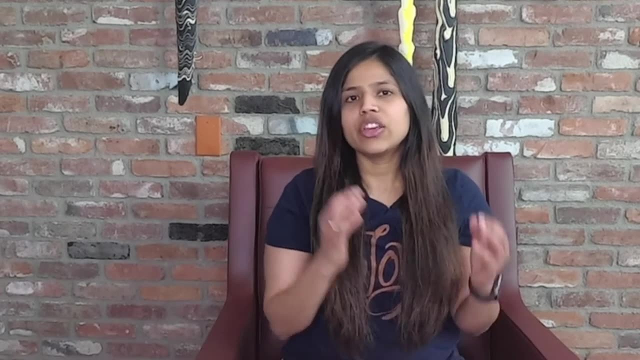 In robotics, this can be how to process sensor data, how to remove noise and how to compute your motor commands to get the robot to move in a specific direction, And that's it. If you know how to code and you can think logically and solve problems. 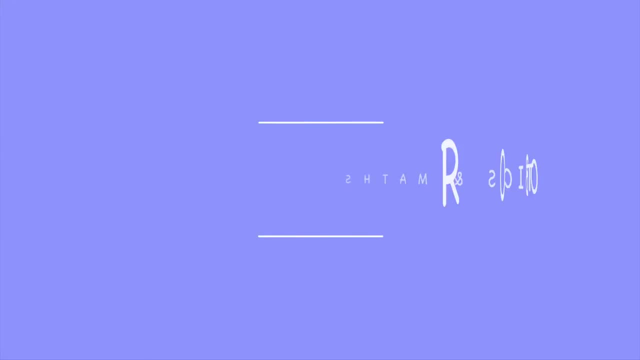 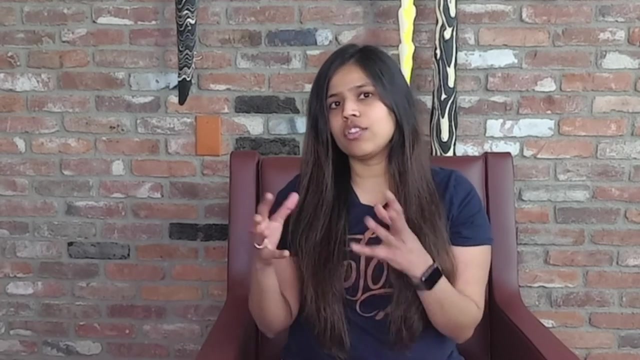 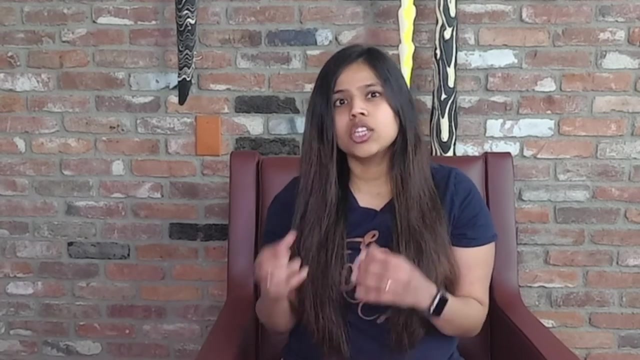 you can do anything you want in the field of robotics. Another topic I want to talk about is math. Now, I know a lot of people out there will say that math is a must for robotics. I disagree with that. Maths, to me, is also a form of logical thinking. 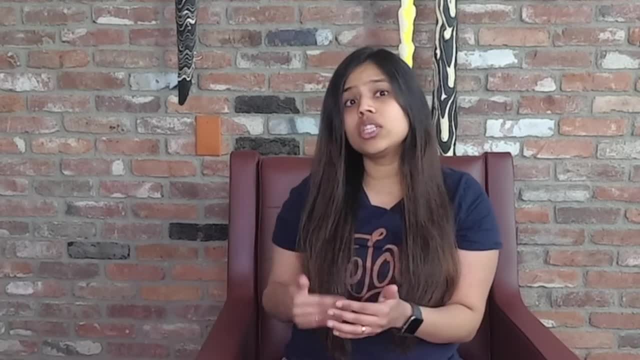 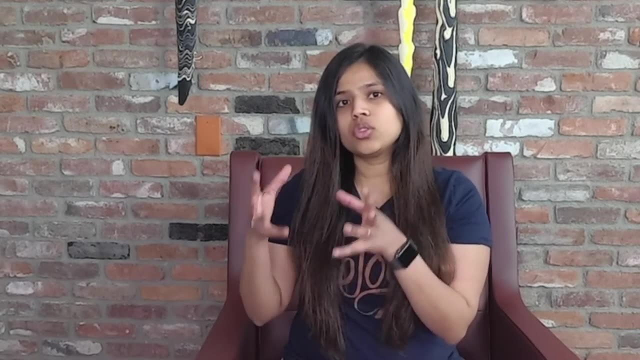 but you don't necessarily need to know math to do robotics. You need to know how to think logically And, just like any other skill, this can also be learned When it comes to solving problems, especially in code. in coding, you can learn how to approach a problem. 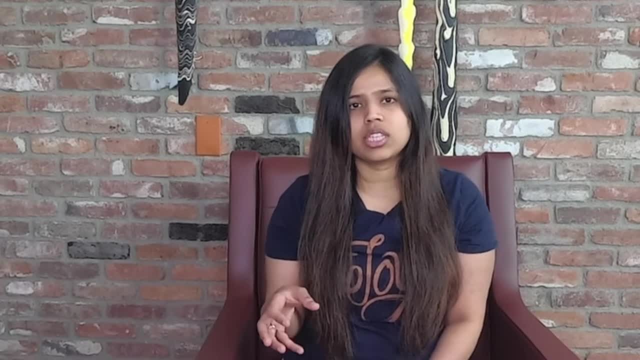 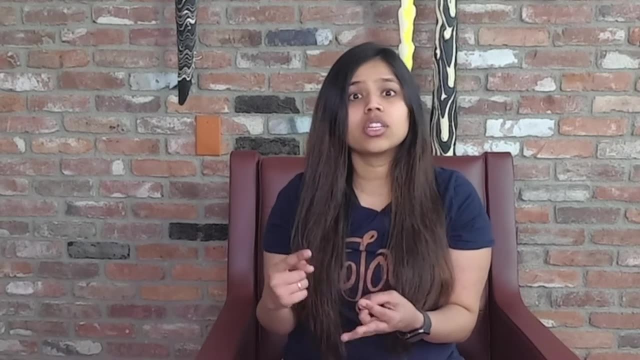 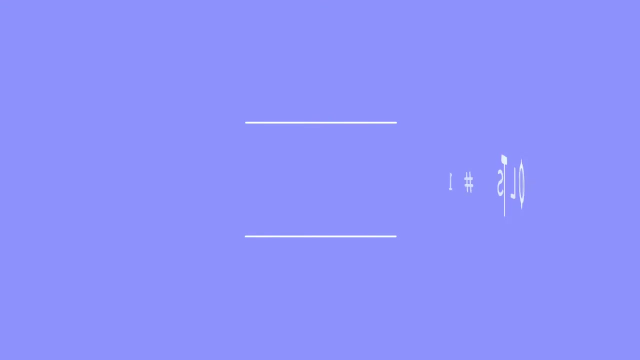 One resource that definitely helped me with this is a course on Coursera called Algorithmic Toolbox. It essentially covers different algorithms, such as greedy algorithm, divide and conquer and dynamic programming, And all of this will help you in terms of how to approach a problem and solve it. 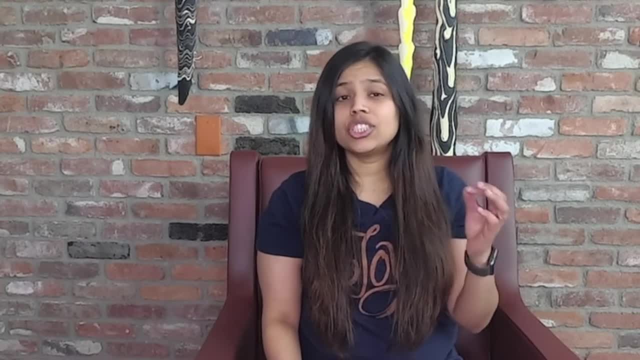 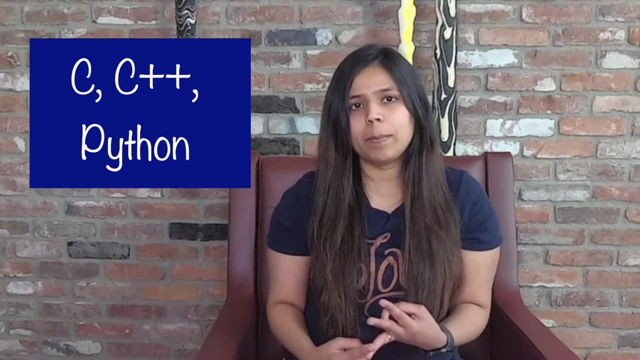 Next let's talk about tools. In the start I mentioned you need programming skills. In terms of tools, this becomes programming languages such as C, C++ or Python. I've seen both C++ and Python used popularly by many robotics companies. 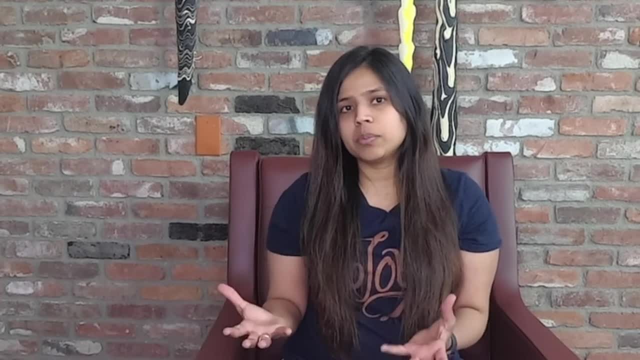 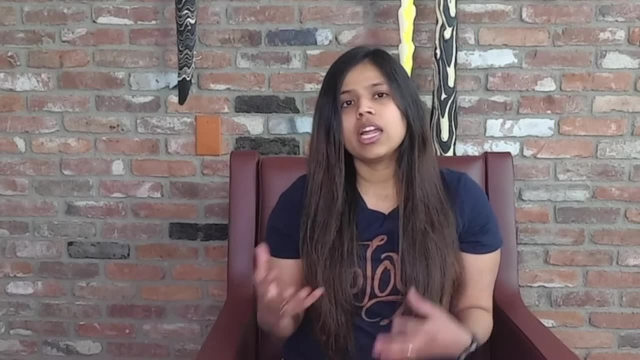 Now, one thing I would like to say is: you don't need to be an expert in both of these programming languages. You can pick one. I would add that get familiar with the second programming language Now. both C++ and Python are object-oriented programming languages. 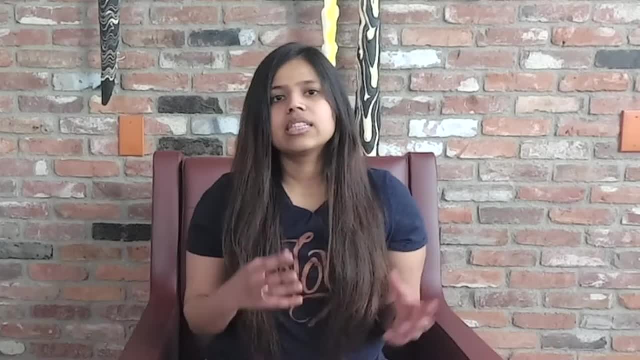 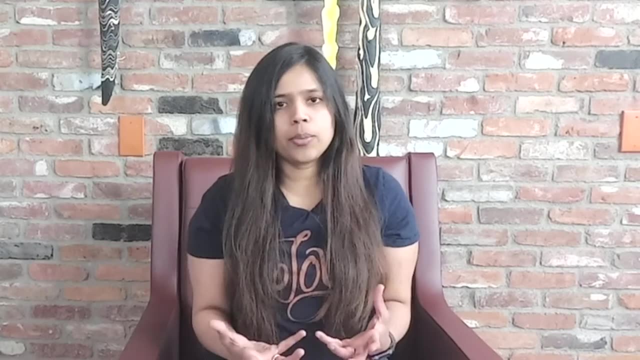 So if you learn one of them, you can easily pick up the other one. The reason I say that get familiar with both of these programming languages is so that you can read other people's code. For example, you're doing a project and you don't necessarily know how to solve it. 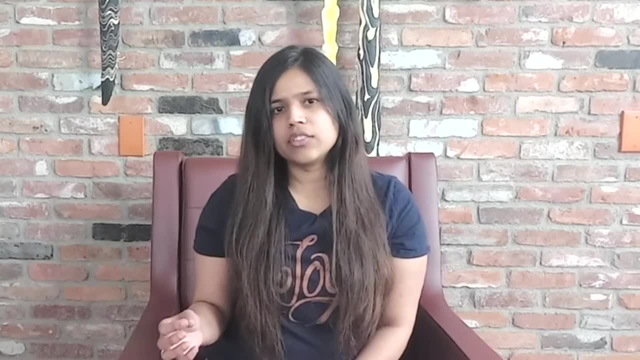 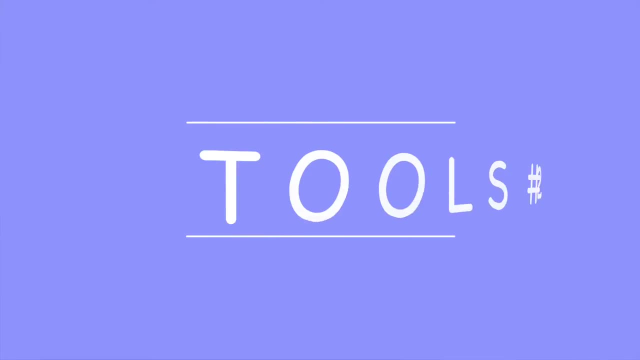 But you find an example online and if you're familiar with the programming language, you should be able to understand the basic logic and replicate it in your programming language preference. Our next tool is ROS Robot Operating System. This has become popular in the recent years. 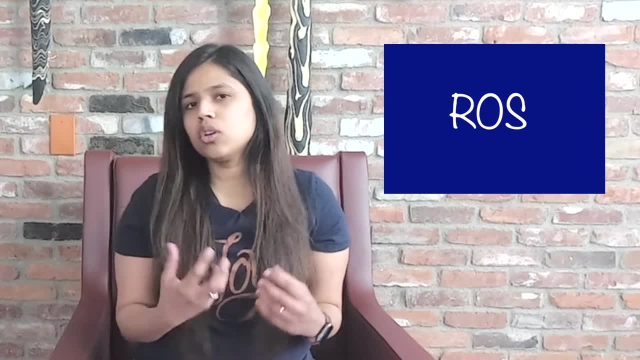 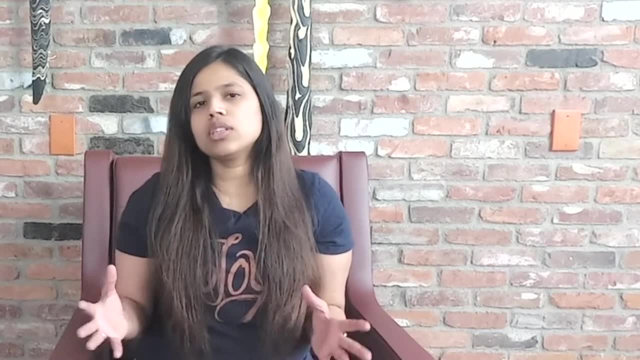 and it makes it easy to work with other people's code. Also, a lot of sensor companies these days have their own ROS nodes, So it's good to know ROS and get familiar with it. You don't necessarily have to spend a lot of time on it. 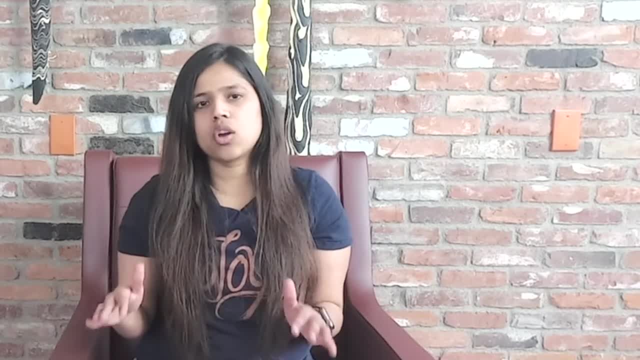 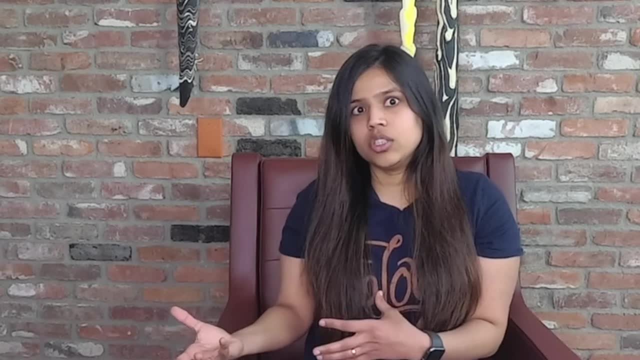 Spend, I would say, a week or two and get familiar with the basic concepts of ROS, which is nodes, topics and services Given robotics. you do have to interact with a robot Now, because I'm speaking from a software engineering perspective. 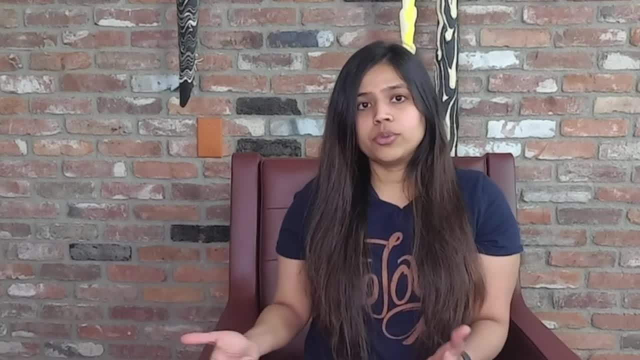 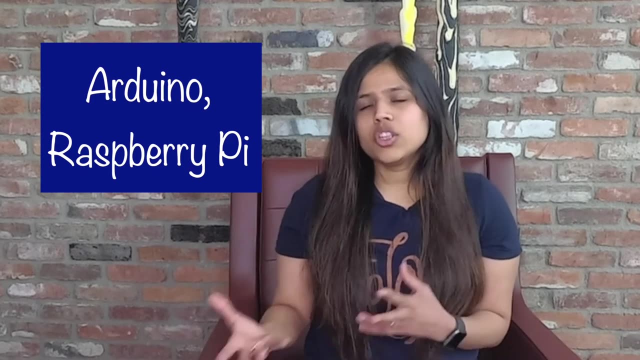 I don't want to talk a lot about hardware, But there are a lot of options. if you want to get started, There's Arduino and Raspberry Pi, or you can even take up any microcontroller and get started. Another option is simulation software. 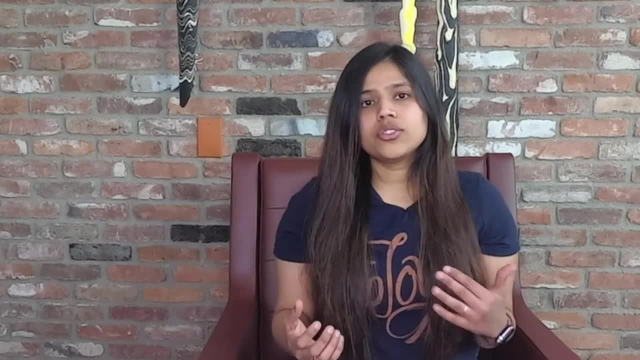 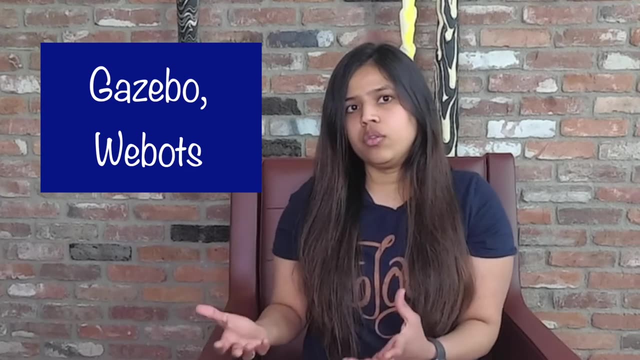 One benefit with simulation software is affordability. Software like Gazebo and WeBots are free, open-source software, so you don't necessarily need to spend, because not everyone can afford different parts, And even with parts such as LIDARs, they can be very expensive. 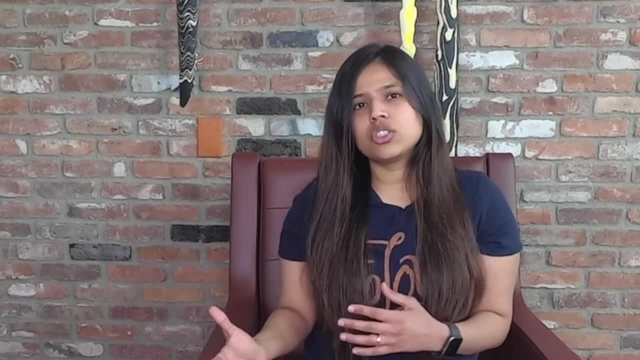 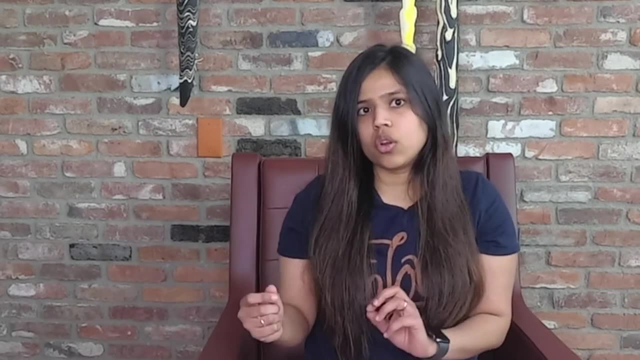 and make it difficult for you to enter. In this case, working with simulation software makes it easy for you to interact. The one thing I would say while using simulation software is: make sure you account for noise Now, with the real-world sensors. 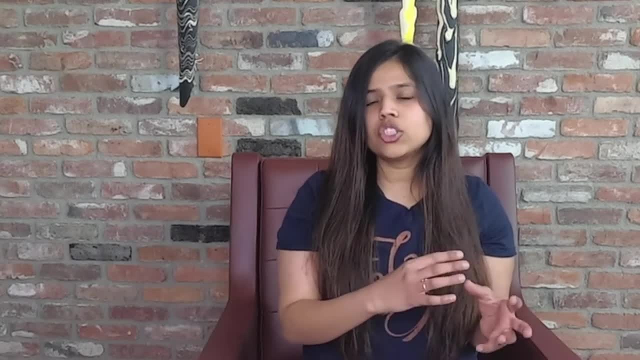 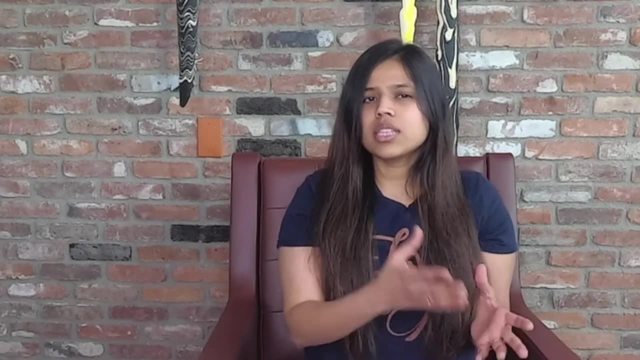 you're going to encounter noise. So when you're working in simulation, make sure you know that there's an ideal world and there's a world with noise. So you have to add some sort of controls to deal with noise. Some softwares have noise inherently. 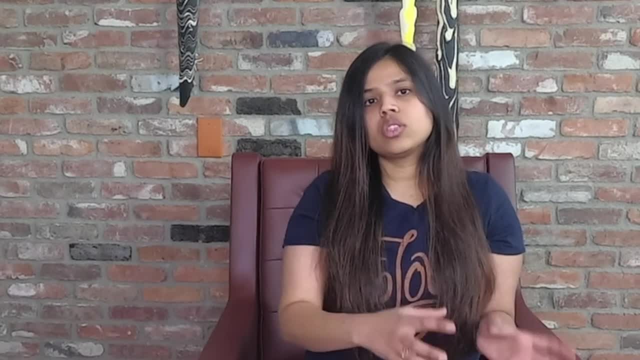 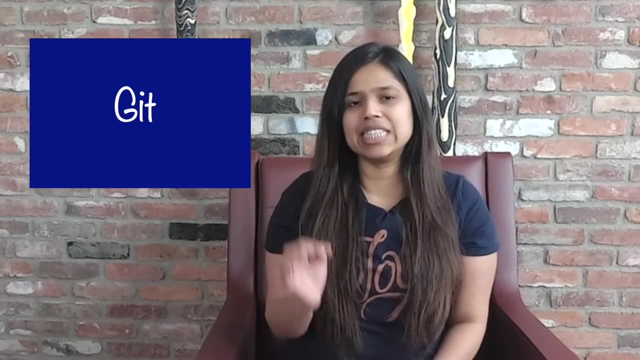 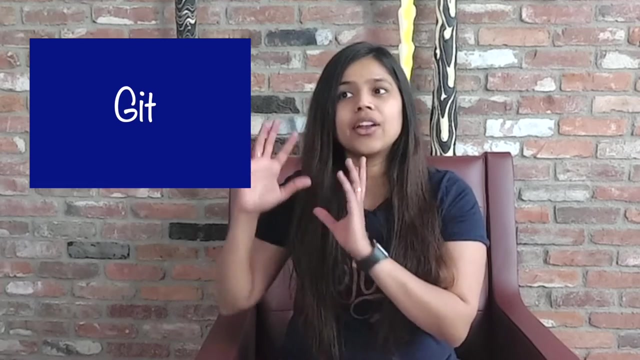 With some softwares, you have to make sure to add noise so that it represents a real world. Another useful tool in robotics or any software engineering position is Git. Git can be used to control versions, as well as to create your own brand and work on your code and not mess up the main code. 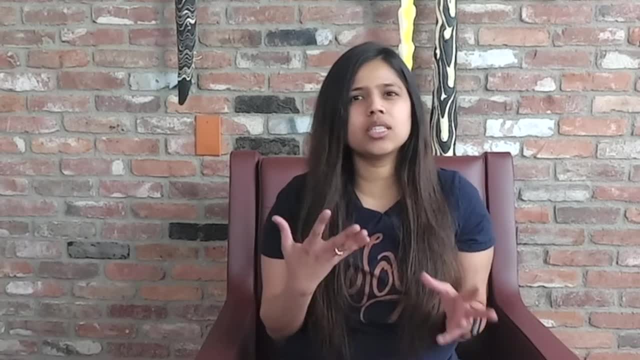 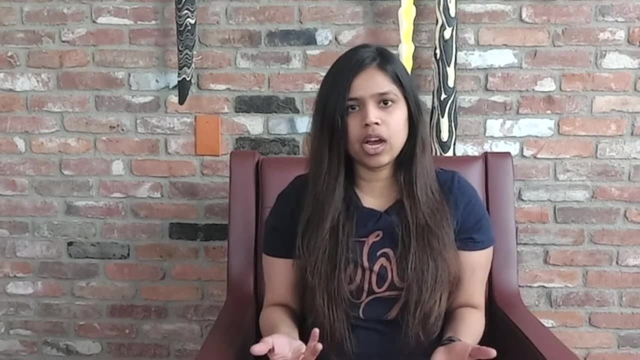 Again, this is a tool that can be picked up fairly quickly. You can either spend a day or week and get familiar with it Now. if you're a student, I would highly encourage you start using Git from now for your assignments and projects. 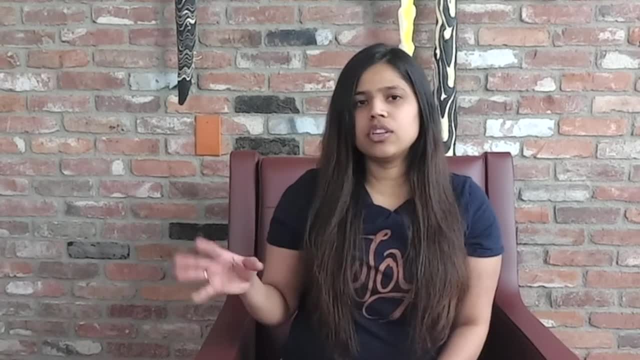 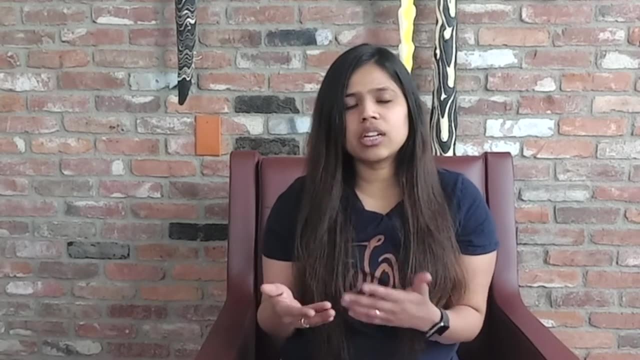 Create a GitHub profile and start pushing your code. This way, you would have also created a portfolio for yourself. I would add that make sure to add documentation and if you've done any images or videos, also upload. This way, it can become a portfolio. 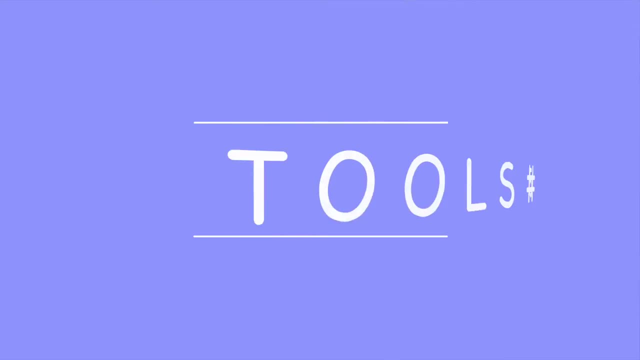 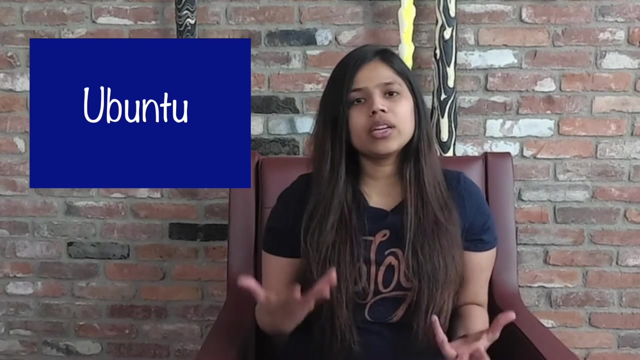 where someone can see what you have done. Before I talk about the next one. I want to talk about OS operating system For robotics. learn to use Ubuntu Now. I grew up in India, so I know in schools and colleges Windows is much more popular, followed by Mac. 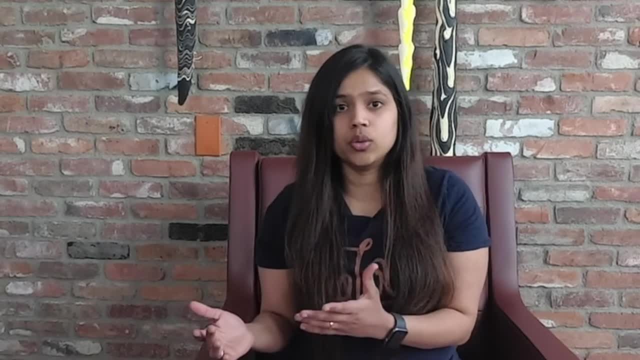 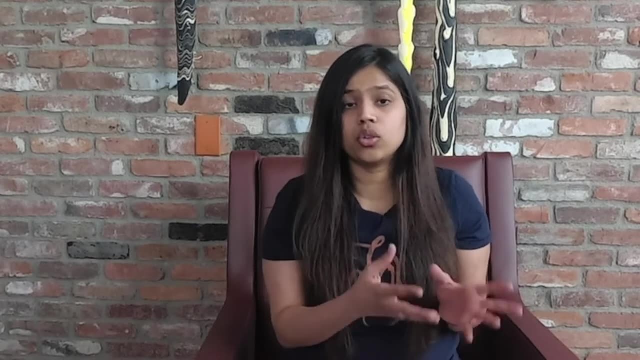 But if you are serious about robotics, learn to use Ubuntu Now. you don't have to necessarily buy a new computer or a laptop. Ubuntu is a free, open source software, so you can download it onto your computer. You can choose to create a partition that way. 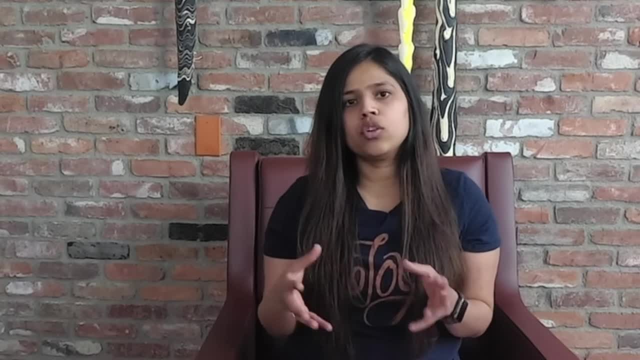 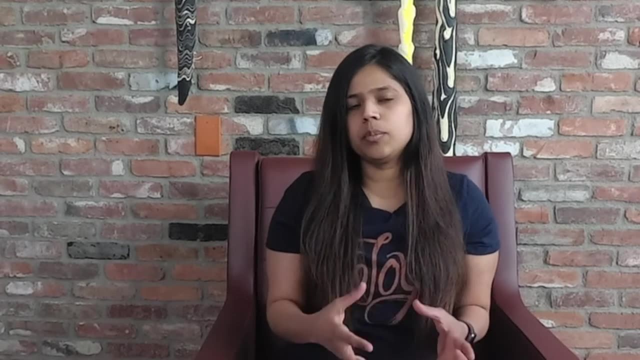 you can have multiple operating systems on your computer. Just be mindful of the fact that it will take up a lot of your memory space. Now, the reason I say get familiar with Ubuntu is because most of the people in the field of robotics use Ubuntu. 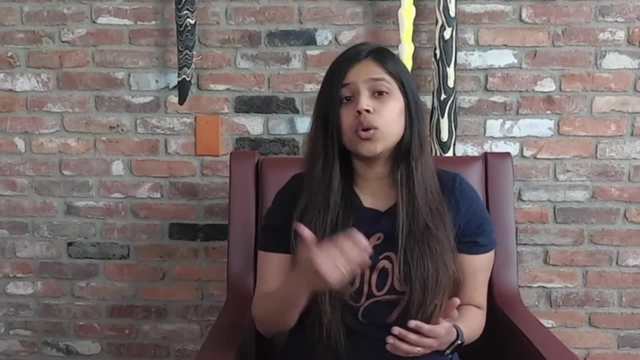 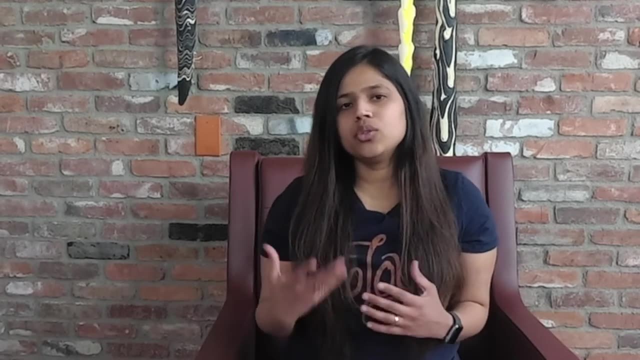 So even when you go in the industry and start working with a company, you're more than likely to be using Ubuntu. Next, a lot of resources are also available for Ubuntu. For example, you want to use Python 3 for ROS And if you Google it, you'll find more resources for Ubuntu compared to Windows. 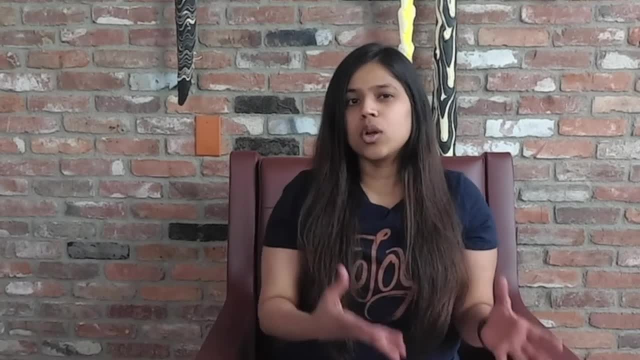 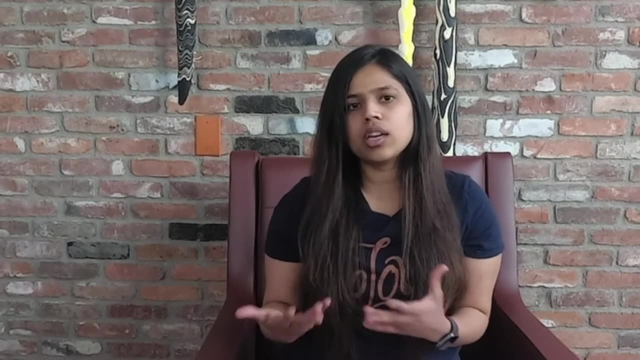 And this is something you'll see with all the other softwares as well. Because most people are using Ubuntu, most answers and resources will be available for Ubuntu. Again, it doesn't require a lot of time. If you spend a week or so, you will start to become familiar with it. 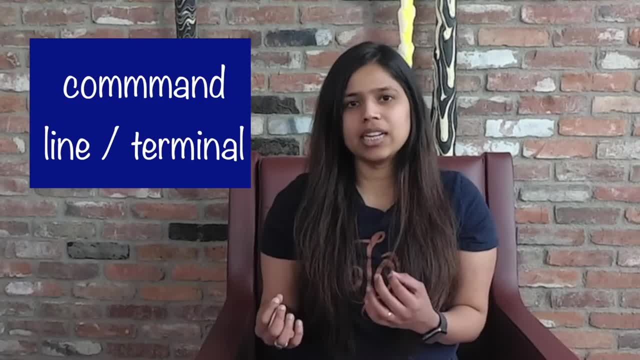 With that, the tool I want to talk about is command line. Get familiar with using command line. Again. this is something you don't necessarily need weekly. You can use it for a lot of things. You can use it for a lot of things. 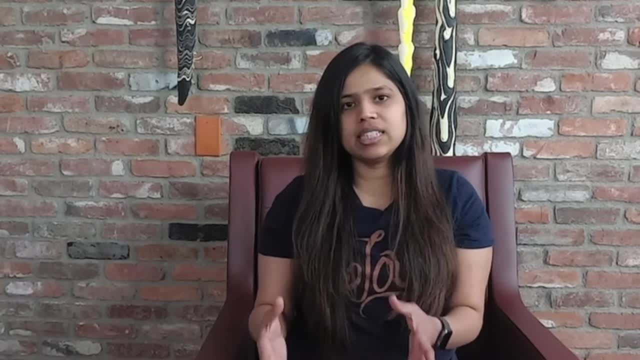 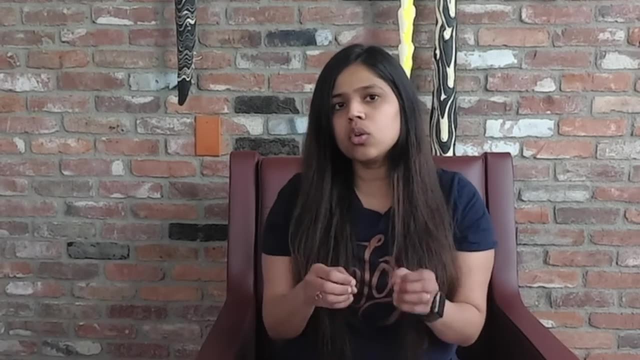 You can use it to learn. Spend a day or week and you can easily start using command line. The reason I say this is when you're working with your projects and you're trying to debug code, you don't always look into an editor. 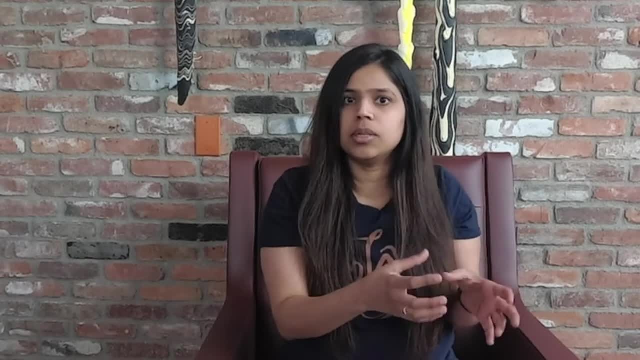 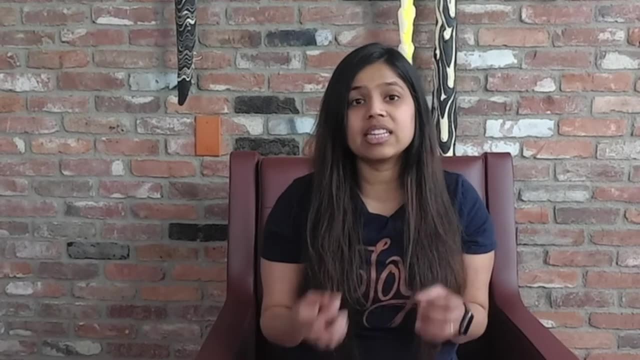 If you're connected to a robot, it's more likely that you just have a terminal to access the code and debug it. So learn how to use command line to move files, copy files and even edit your code. Learn some command line editors, such as VI or VIM, so that you can easily debug your code. 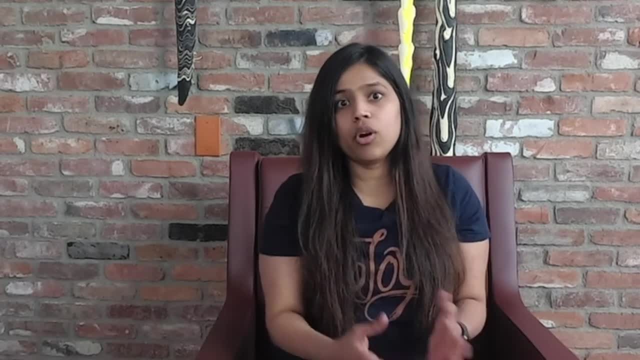 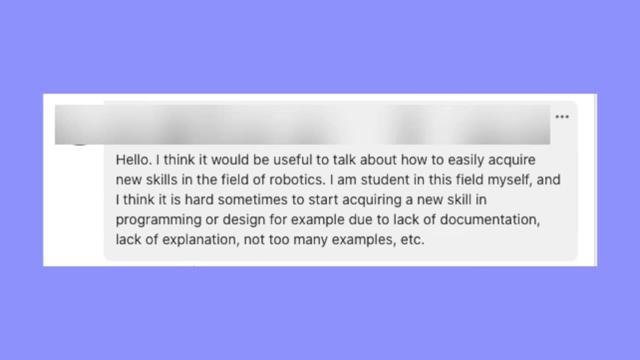 Learn some command line editors, such as VI or VIM, so that you can easily debug your code code when you're connected to a robot and don't have access to an editor. An interesting question I received is the following. I think it would be useful to talk. 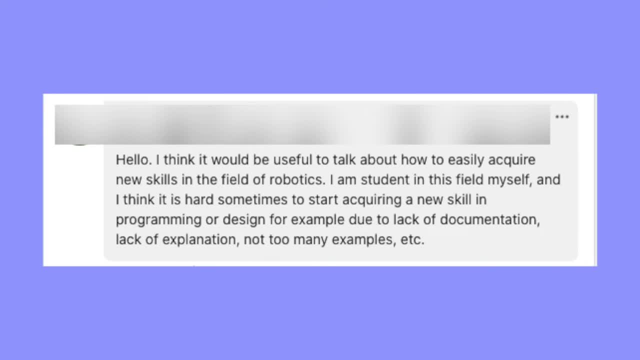 about how to easily acquire new skills in the field of robotics. I'm a student in this field myself and I think it's hard sometimes to start acquiring a new skill in programming or design, for example, due to lack of documentation, lack of explanation, not too many examples, etc. 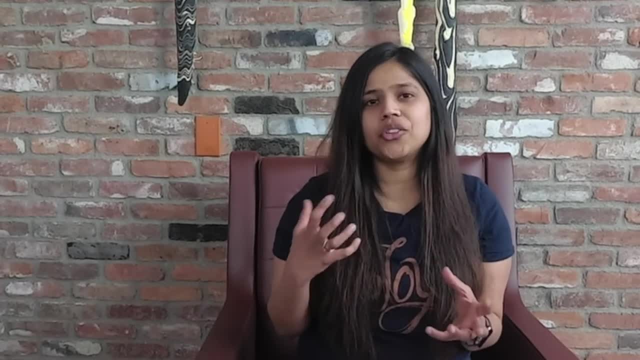 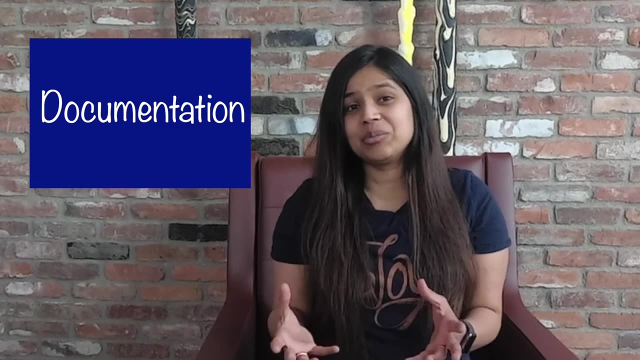 I agree with the last statement. There isn't a lot of documentation or example when it comes to robotics. Now, one, robotics is a growing field and second, documentation is kind of that task that you need to do but nobody really does it because it's boring. Now, if you yourself imagine, 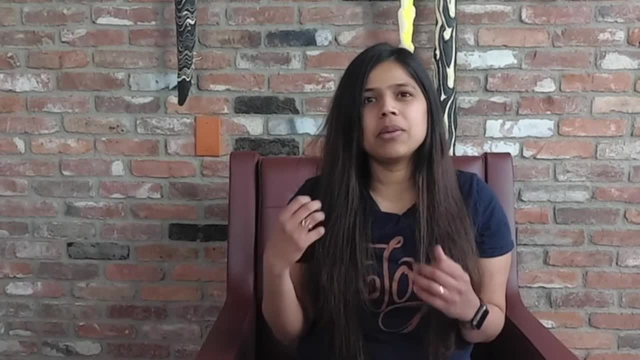 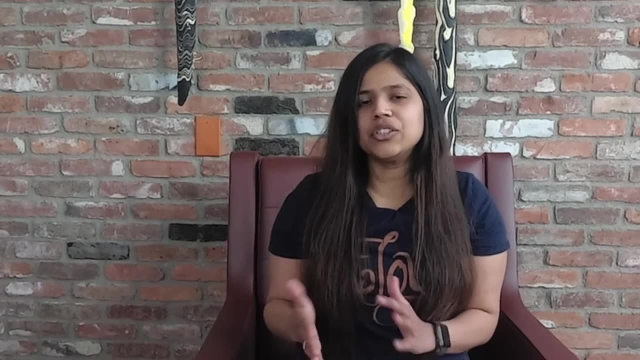 especially as a student. you started doing your assignments maybe a week or a day before the deadline and you never really thought about writing documentation. The same is kind of true in the industry as well. You're always working on your assignments and you're always 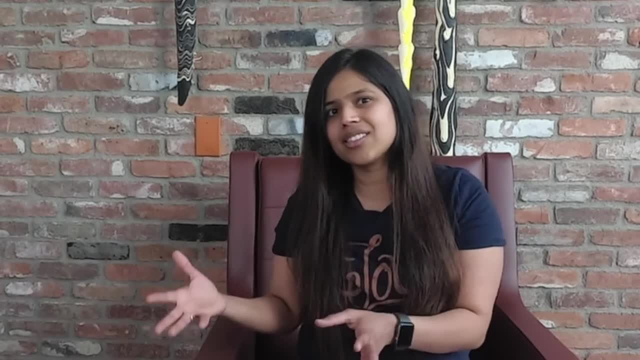 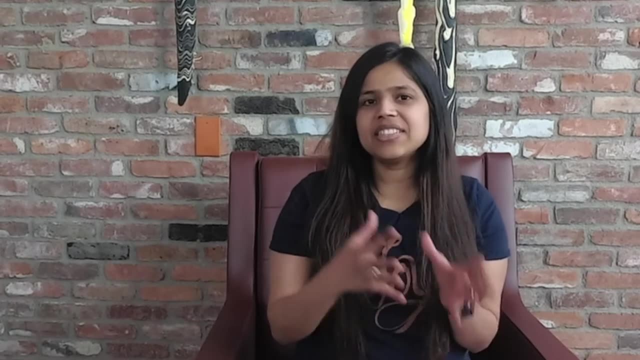 working on lots of these tasks and documentation is the last thing to be done, but before you get to it, either something else comes up or, because it's boring, you don't really do it. Having said that, acquiring skills in robotics is not necessarily easy, and you have to get your. 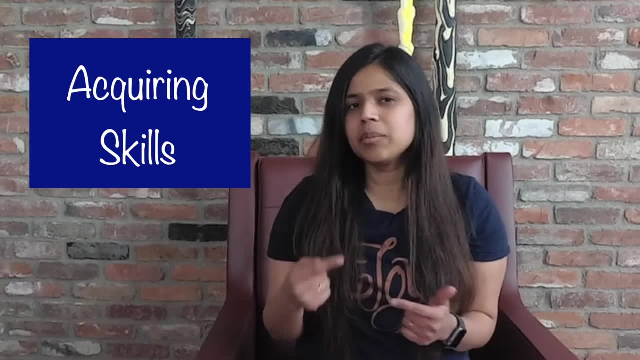 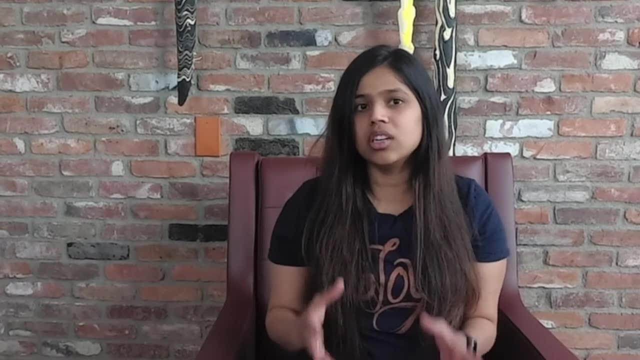 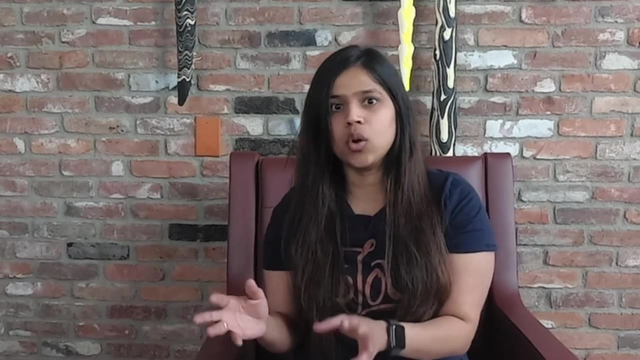 hands dirty. Now, if you look at some of the interviews that I've conducted, time and again, everyone gives the same advice: Get your hands dirty and do a robotics project. That's the best way to learn and acquire new skills in robotics. The thing is, robotics is not something where you pick an algorithm and apply it and hope. 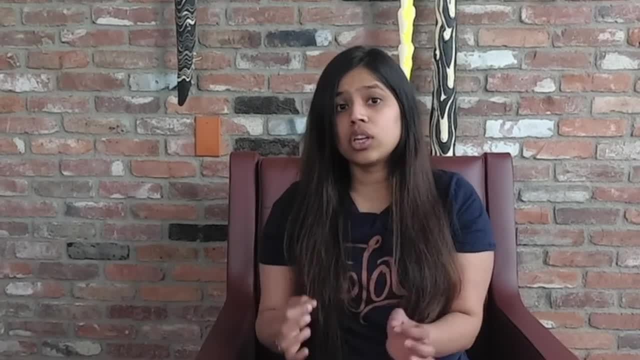 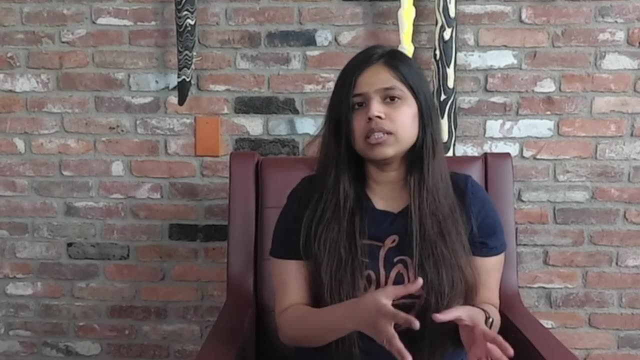 for it to work, You really have to understand and tweak it for it to work with your particular set of environment and robot. So, for example, take a line following robot. The algorithm in itself is very simple, but if you copy and paste it it might not work for you. For example, 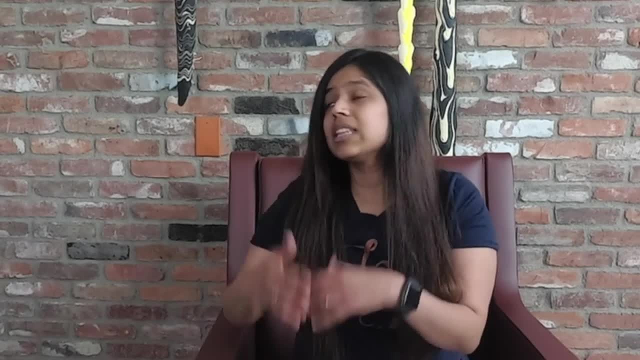 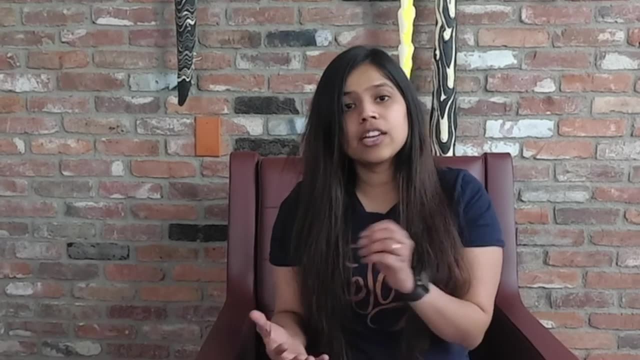 the color of your line for the line follower might be different, The ambient light, that is, the light around you, might be different, causing the light reflected by the line to be different, and your sensor might not detect the line. So you might have to tweak those. 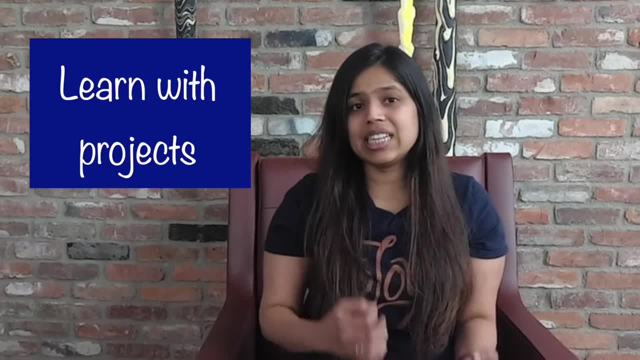 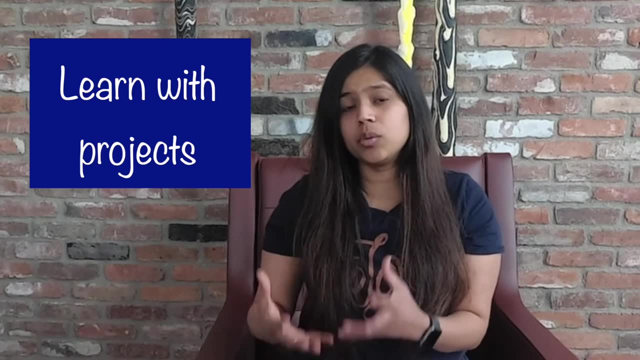 things for the line to be detected. All I'm trying to say is it takes time and you have to get your hands dirty to really learn the skills. Giving a personal example, it definitely took me a lot of time to get started with the basics, Even coding. it wasn't that easy. 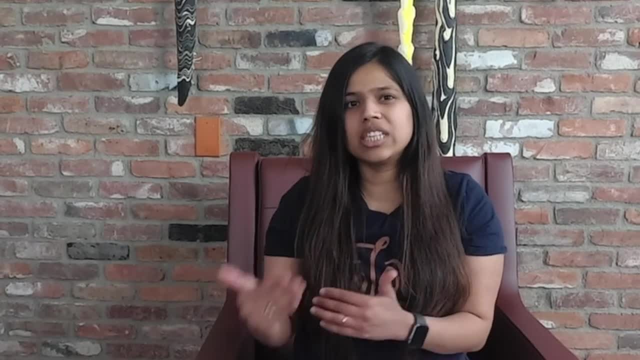 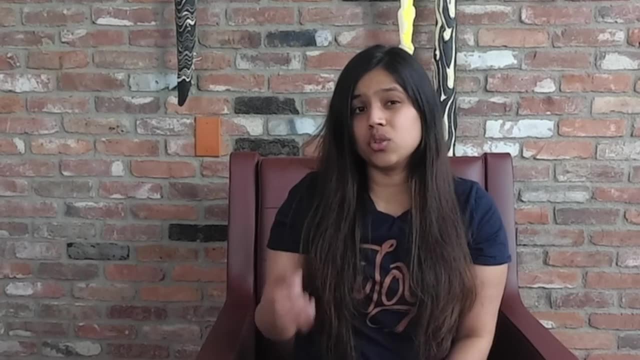 and it took me a while before I got good at it. So make sure to give yourself that time and invest in learning those skills. Apart from projects, another useful avenue is robotics. The reason I say robotic competitions is because the goal is already decided and there are. 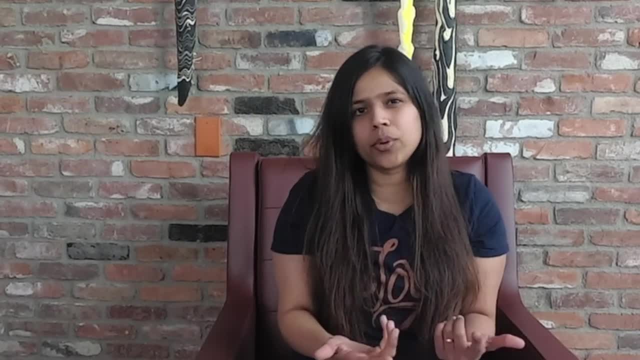 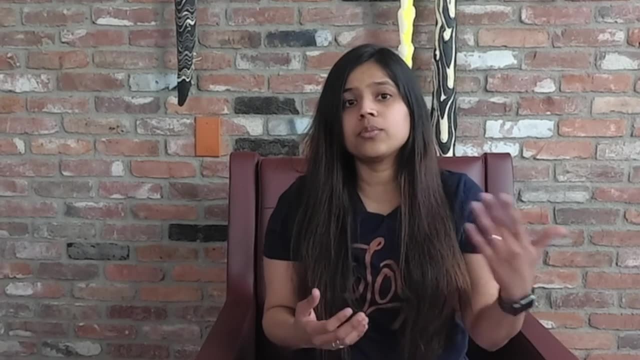 concrete deadlines which make sure that you continue working on your project and not get demotivated. Plus, you're working as a team, so you can help one another and also get help from seniors or the community surrounding the competition. Another question I received: 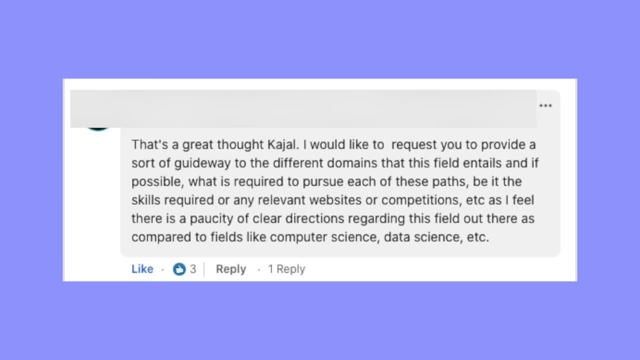 was. I'd like to request you to provide a sort of guide way to the different domains that this field entails or, if possible, can you provide a guide way to the different domains that this field entails and, if possible, can you provide a guidance to those that you don't?